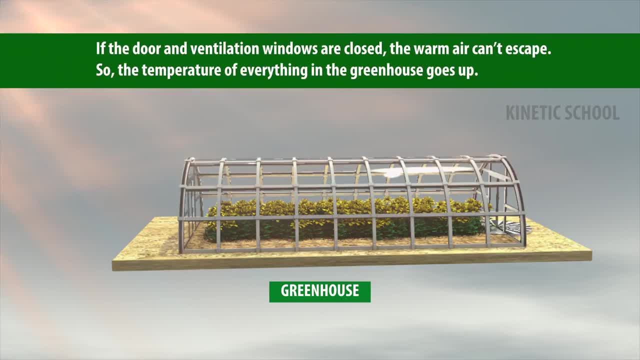 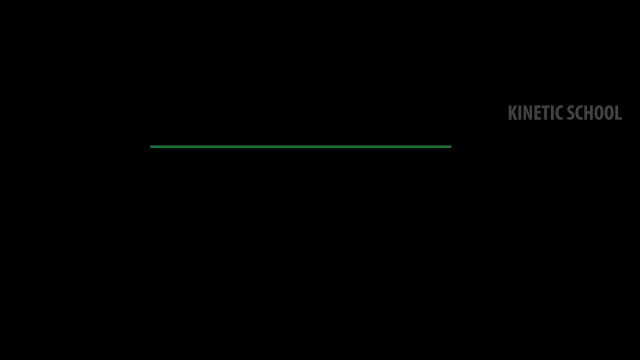 If the door and ventilation windows are closed, the warm air can't escape, so the temperature of everything in the greenhouse goes up. Thus greenhouse acts as a heat trap. Electromagnetic Spectrum: An shortwave, longwave radiation. 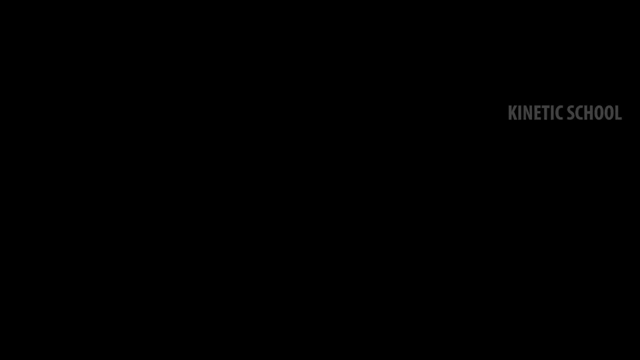 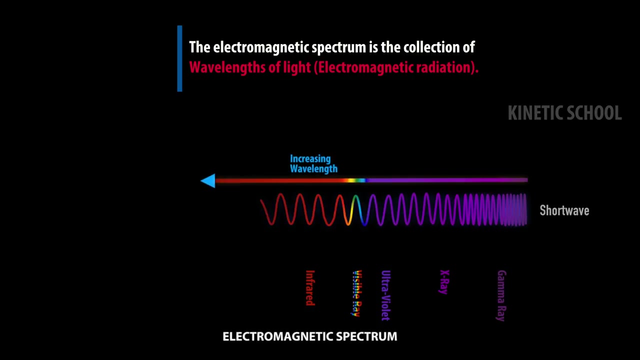 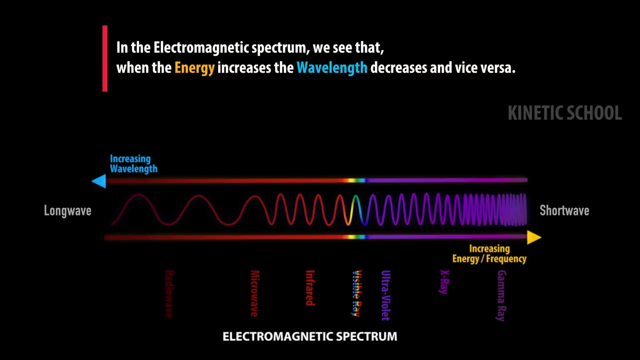 passed through the lavalier clan against human radiation, ft. Everything that has a temperature gives off electromagnetic radiation. In the electromagnetic spectrum we see that when the energy enters the lavalier homes are increases, the wavelength decreases and vice versa. 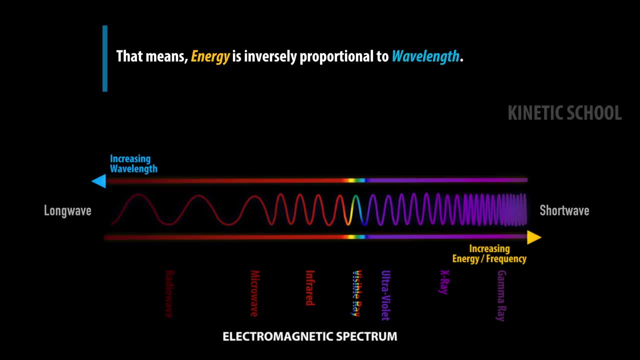 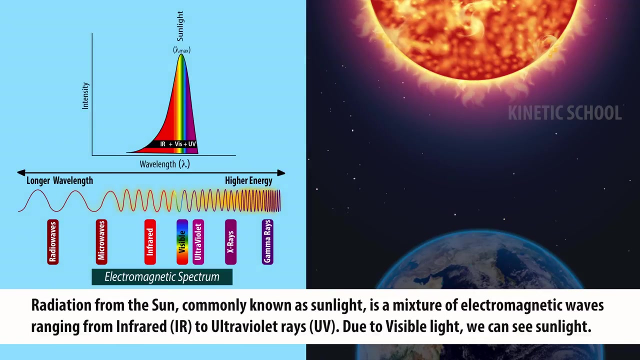 that means energy is inversely proportional to wavelength, so short wave radiation contains higher amounts of energy, and long wave radiation contains a smaller amount of energy. radiation from the sun, commonly known as sunlight, is a mixture of electromagnetic waves ranging from infrared to ultraviolet rays due to visible light. 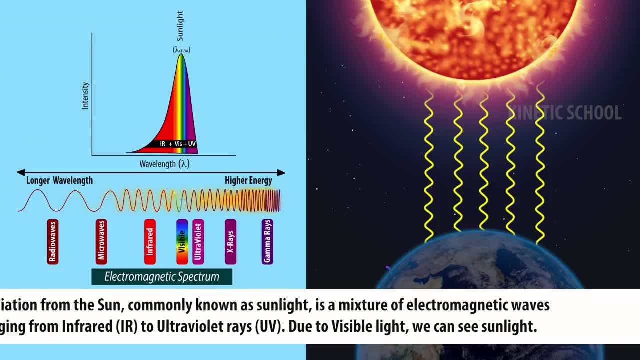 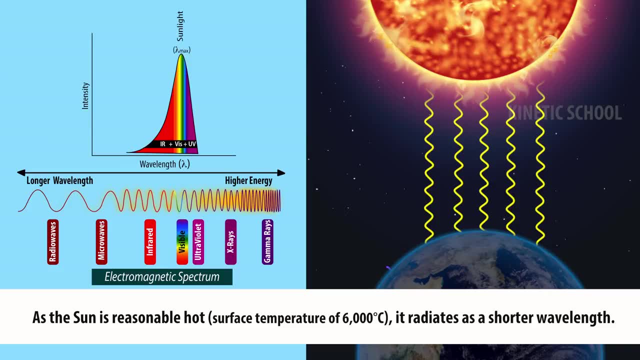 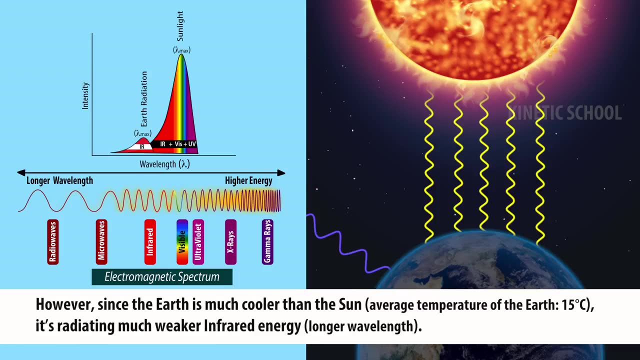 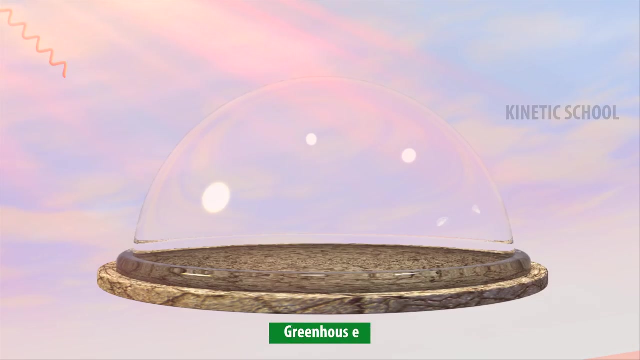 we can see sunlight. as the sun is reasonable hot, it radiates as a shorter wavelength. however, since the earth is much cooler than the sun, it's radiating much weaker infrared energy. how greenhouse works, solar energy enters our atmosphere as short wave radiation in the form of 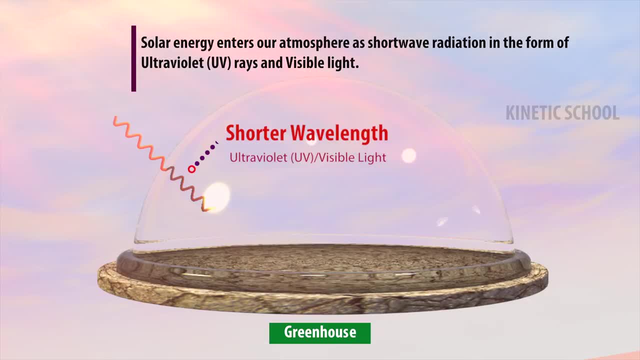 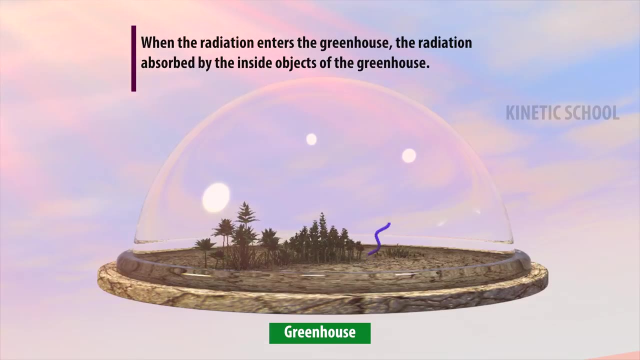 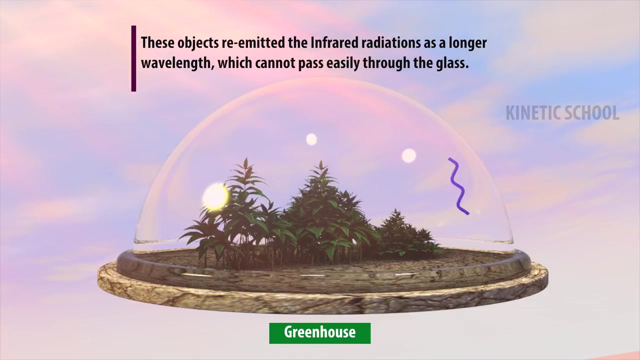 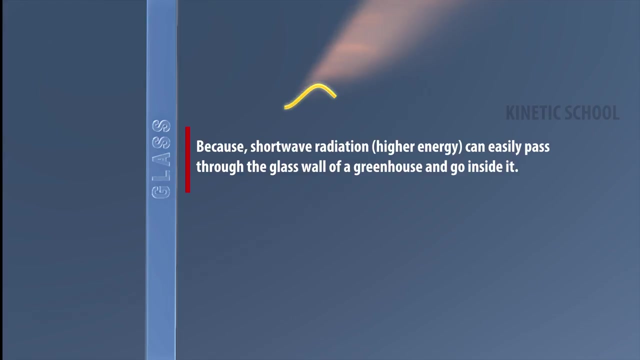 ultraviolet rays in visible light. when the radiation enters the greenhouse, the radiation absorbed by the inside objects of the greenhouse. these objects re-emitted the infrared radiations as a longer wavelength which cannot pass easily through the glass, because short wave radiation can easily pass through the glass wall of a greenhouse. 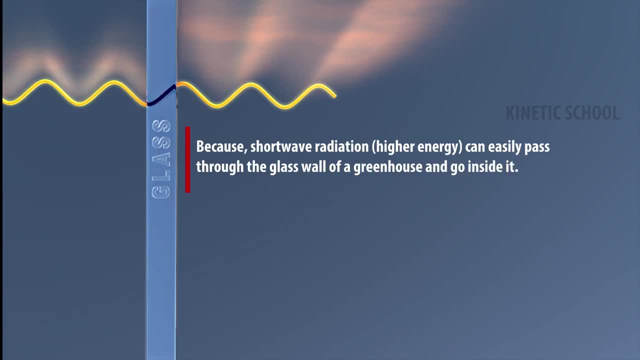 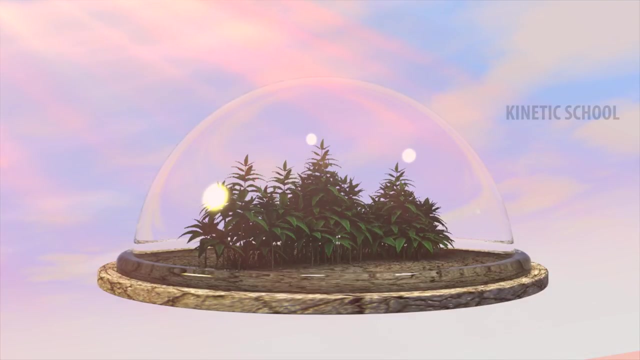 and go inside it, but the longer wavelength radiation does not allow to escape through the glass, so it again reflected inside the greenhouse. but the longer wavelength radiation does not allow to escape through the glass wall of a greenhouse, because short wave radiation can easily pass through the glass wall of a greenhouse. 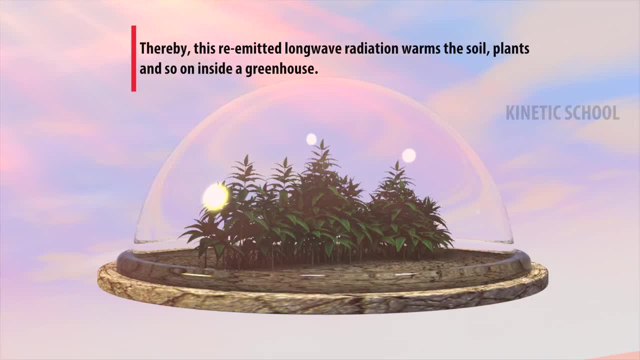 where the air goes to the glass wall, a greenhouse. thereby this re-emitted long wave radiation warms the soil, plants and so on inside a greenhouse. even without an internal supply of heat, the temperature inside a greenhouse becomes higher than that outside. thus the glass acts as a cold source of heat. 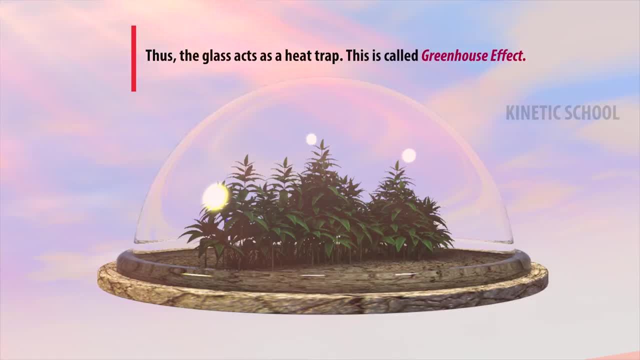 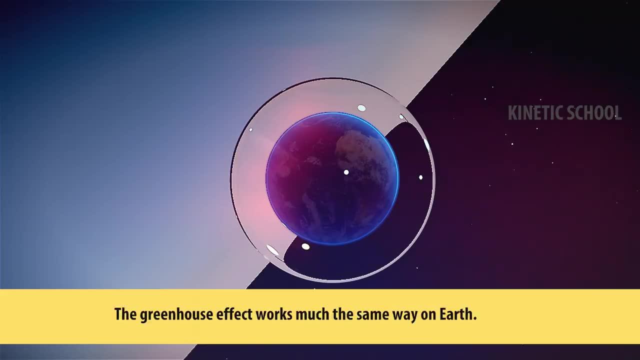 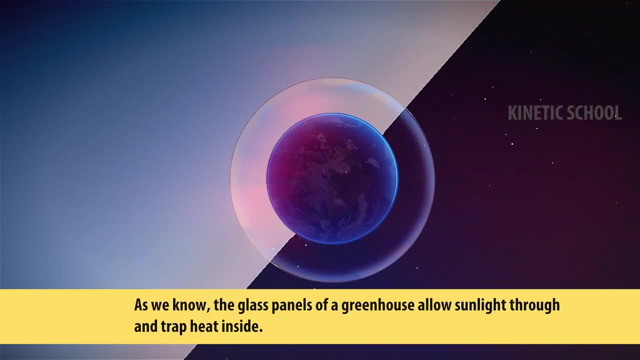 and is a good source of heat for long-wave radiation as a heat trap. This is called greenhouse effect. The greenhouse effect works much the same way on Earth. As we know, the glass panels of a greenhouse allow sunlight through and trap heat inside. 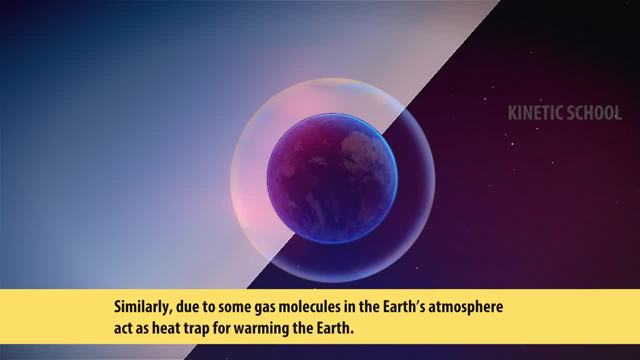 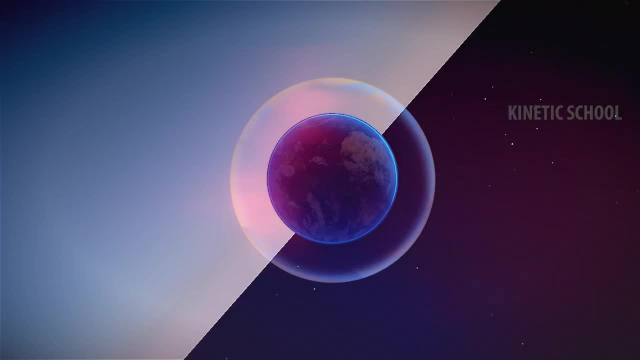 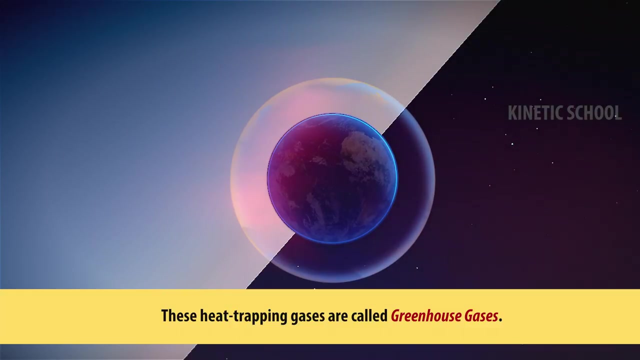 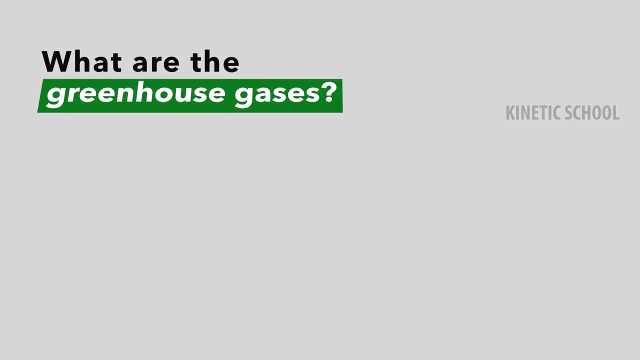 Similarly, due to some gas molecules in the Earth's atmosphere, act as heat trap for warming the Earth. These heat trapping gases are called greenhouse gases. What are the greenhouse gases? Greenhouse gases are the gases that absorb infrared radiation which emitted from Earth's. 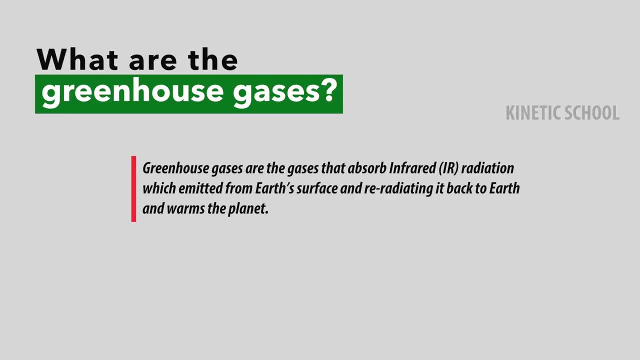 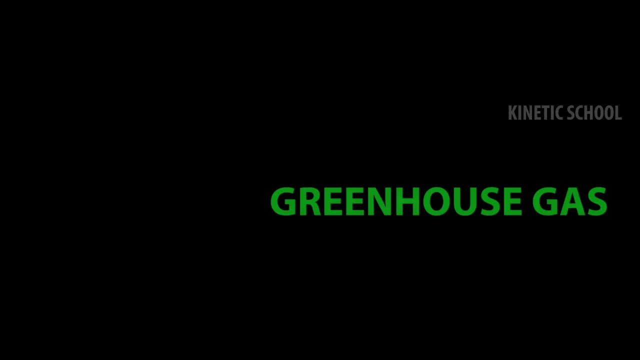 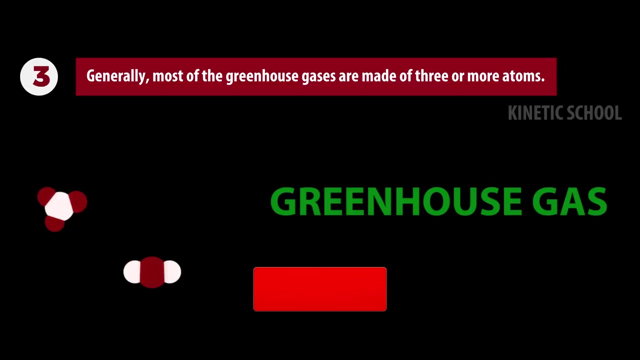 surface and re-radiating it back to Earth and warms the planet. Properties of Greenhouse Gas. Greenhouse gases are transparent to most short wave energy from the sun. Greenhouse gases absorb long wave radiation. Generally, most of the greenhouse gases are made of three or more atoms. 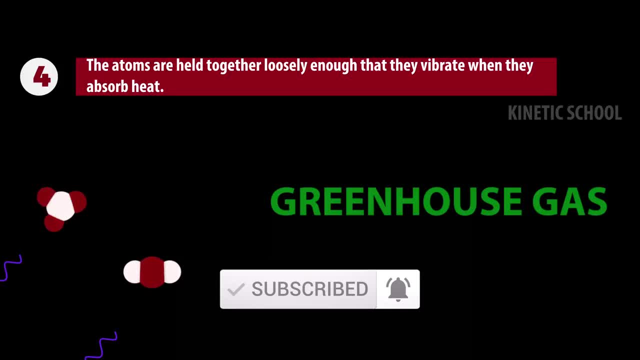 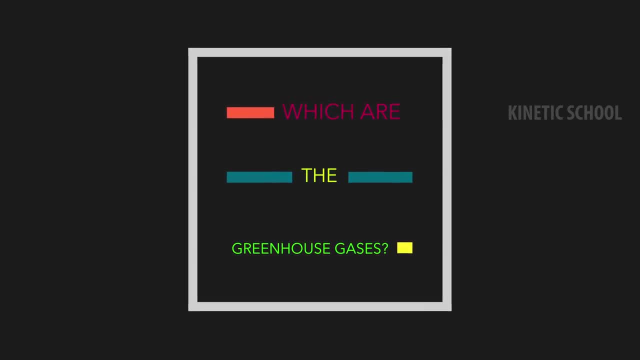 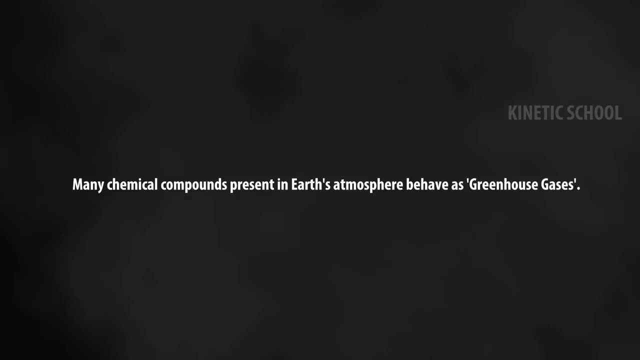 The atoms are held together loosely enough that they vibrate when they absorb heat, Which are the greenhouse gases. The greenhouse gases are stored in seesawšes of used alcohol, Which are the greenhouse gases. The greenhouse gases are stored in theidences. 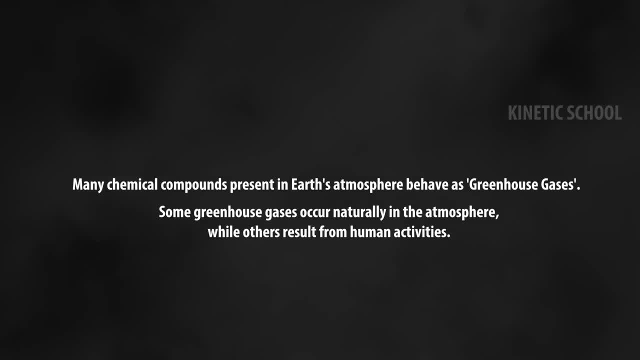 Which are the greenhouse gases. The greenhouse gases: they are requested thanks to theosophic elements of the concerns of the forces that make them act. The greenhouse gases are part of the Poros's process that forecast and estimate the motion of a record time by looking at all glass panels. 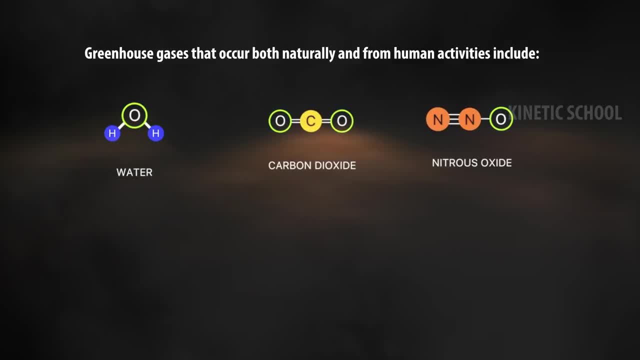 These are basically the greenhouse gases, but there are different classes of the greenhouse gases. Some greenhouses causes natural action and first they have to kill gas. Many of these Indian Ozone, Methane, Chlorofluorocarbon or CFC. 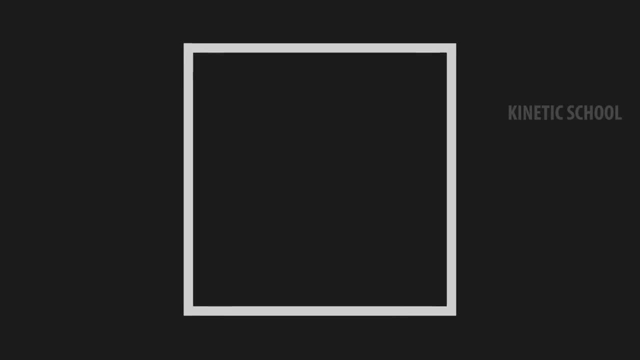 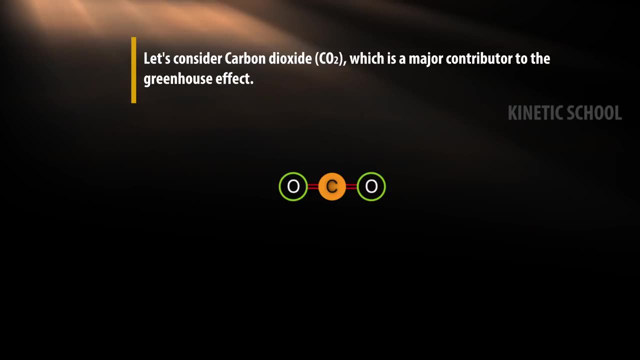 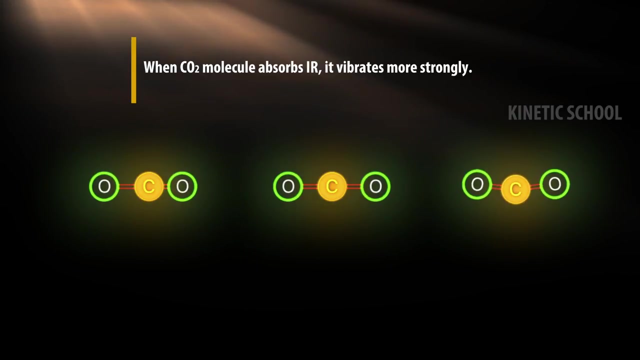 Mechanism of Greenhouse Gases. Let's consider Carbon Dioxide, which is a major contributor to the greenhouse effect. Carbon dioxide is transparent to visible light but absorbs infrared radiation. That means infrared radiation cannot pass through the carbon dioxide. When carbon dioxide molecule absorbs infrared, it vibrates more strongly.